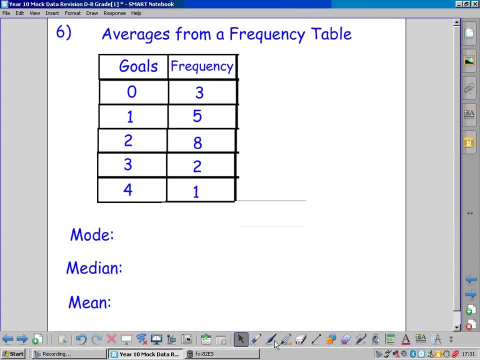 Finding averages from a frequency table should be fairly straightforward. The mode is the one that comes up the most. I've got a frequency table. The frequency that comes up the most is 8, but that's not the mode. The mode, or number of goals, is what we're after, not the 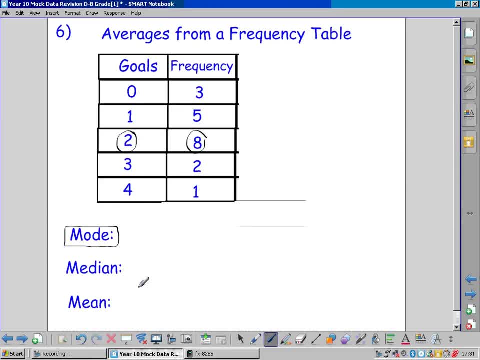 number that comes up the most. That indicates that it's two goals. that's the mode. The most common number of goals per game is 2,, not 8.. The median requires two steps of working out. To find the median, we do n plus 1 divided by 2, and n is the number of games. Now these 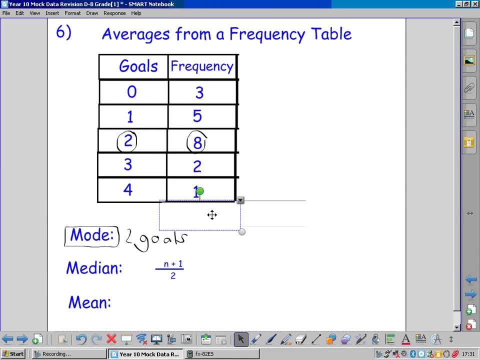 are the goals and these are the frequencies. How do we find the number of games? It's the total frequency. So we add them up: 3 and 5 and 8 and 2 and 1.. Which gives us 19.. So that was 19 games in total. So we do 19 plus 1 divided by 2, which 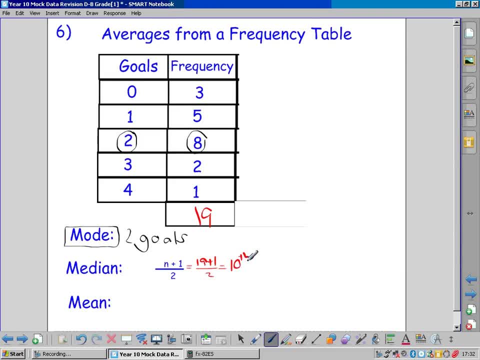 is 20 divided by 2, which is 10.. So we want to find the score in the tenth game. Where's the tenth game? We need to arrange these in order. in a running total, So 3, 3 plus 5. 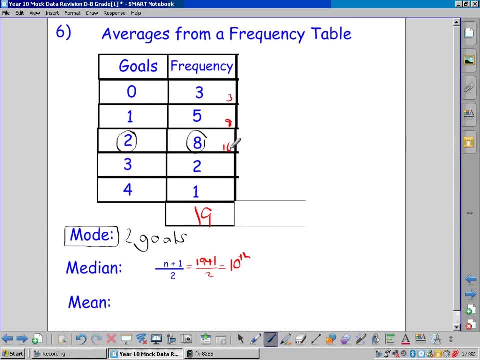 is 8.. 8 plus 8 is 16.. 16 plus 2 is 18.. 18 plus 2 is 16.. 18 plus 2 is 16.. 18 plus 2 is 16.. 18 plus 1 is 19.. Where would the tenth game be? Well, here's the first three games. 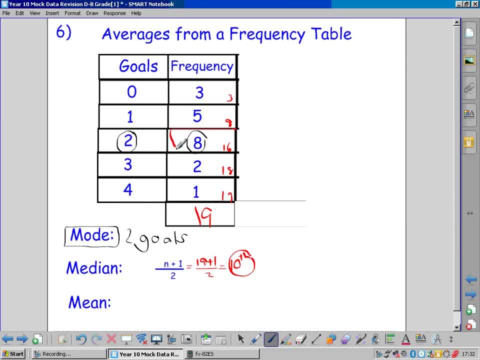 then 8.. The tenth game would be one of these games, with a third game in here, which means the median goals per game is 2.. The tenth game would be in this row, so it would be 2.. So the answer again is two goals, Not 8,, not 10, 2.. 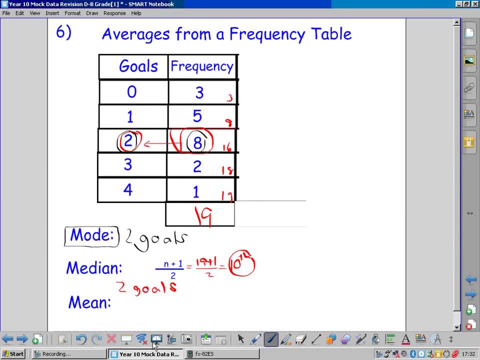 Subtitles by the Amaraorg community. We clear all of that because they're only worth a few marks, whereas the mean from a frequency table could be worth up to four marks. To find the mean in primary school you learn: add up all the numbers and divide by how many there are. So we need to add up.